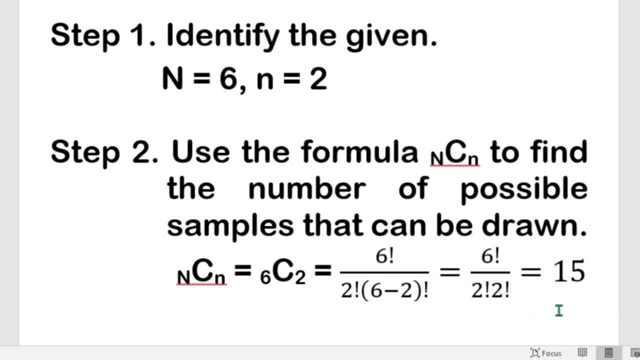 And solving that. we have our solution here. Thus, when we want to determine two samples, there are 415 possible combinations. 10 喜 using our formula 7: 00r is very necessary, especially when we have a larger samples, but in this case we can just. 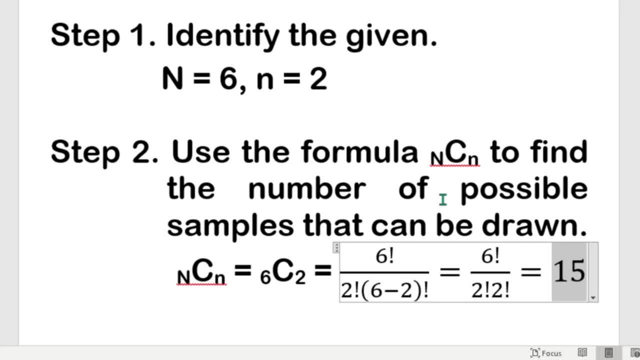 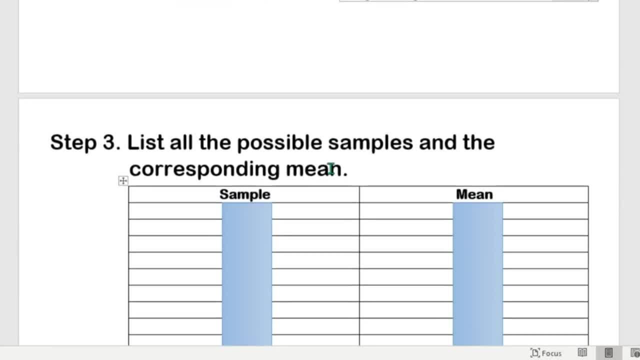 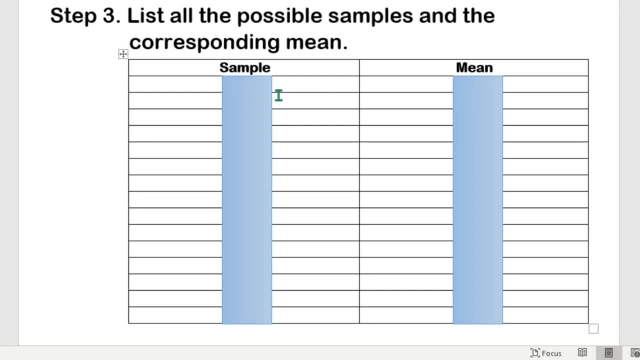 simply proceed to our step number three. but it is better that we know how many possible samples we will have. Let us proceed to step three. Now for the next step. we list all the possible samples on the corresponding mean. Remember that we have six numbers and we draw. 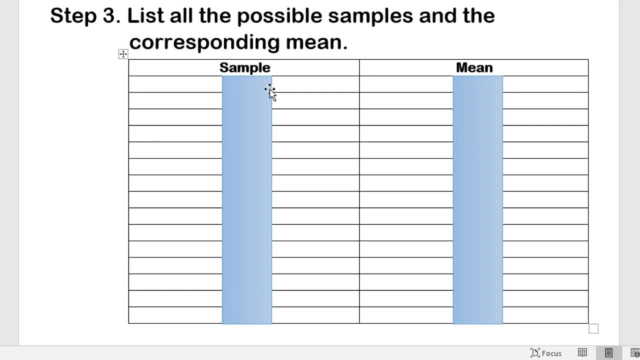 two out of the six numbers and we have the possible samples. It could be 1, 2, 1, 3, 1, 4, 1, 5, 1, 6, 2, 3, 2, 4, 2, 5, 2, 6, 3, 4, 3, 5, 3, 6, 4, 5, 4, 6, 5, 6.. 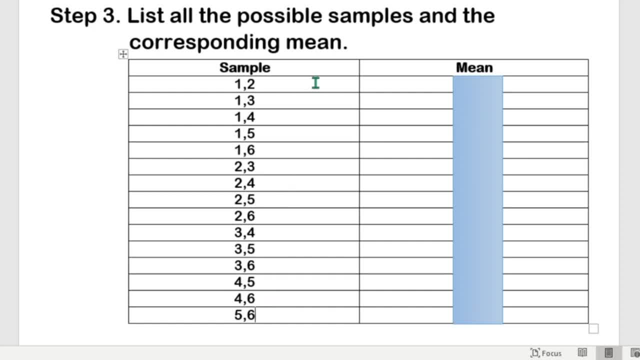 Now these are all the possible samples and we determine the mean of each sample We have for 1, 2, the mean is 1.5, the mean of 1 and 3, the sum of 1 and 3 is 4, divided by 2 is 2. 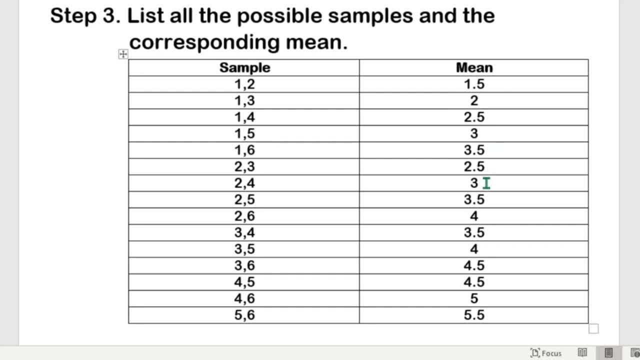 and we have 2.5,, 3,, 3.5,, 2.5,, 3,, 3.5,, 4,, 3.5,, 4,, 4.5,, 4.5 and 5 and 5.5.. 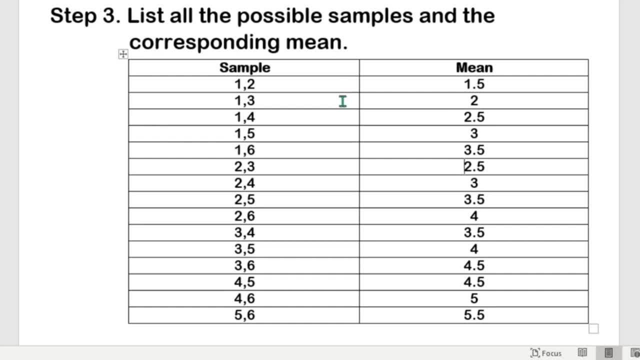 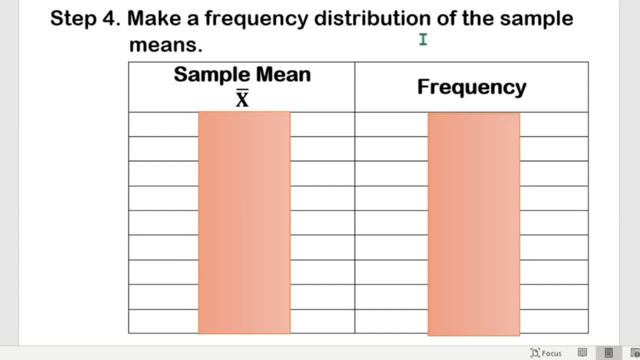 Now we have listed the possible samples and the corresponding mean, To be able to know the sampling distribution of the sample means, we proceed to the next step, which is we make a frequency distribution of the sample means. In this table we only have two columns. The first column are the sample means and the second column are the corresponding frequencies. 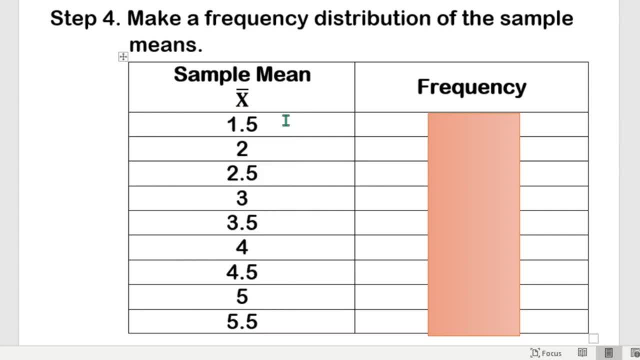 Let us uncover this one Again. we have the sample means: 1.5, 2, 2.5, 3, 3.5, 4, 4.5,, 5 and 5.5.. Where did we get this? We got this from. 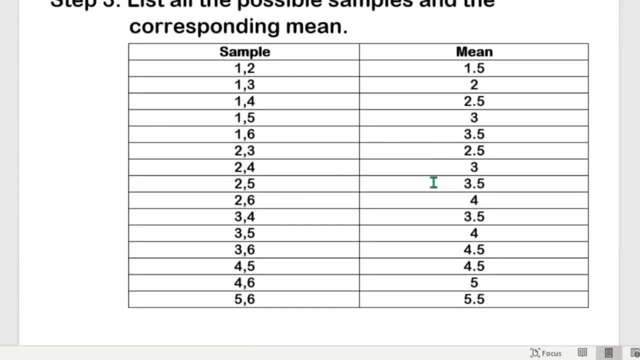 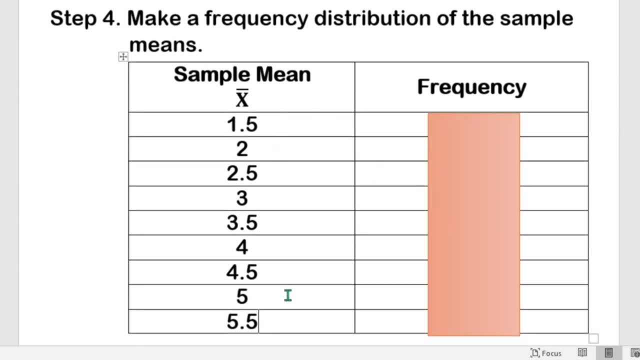 this table that we have and again we determine the sample means and we listed it here- and we determine the frequencies, How many samples we have a mean of 1.5, we have 1, with a mean of 2, we have 1, with a mean of 2.5 is 2, with a mean of 3 is 2, with a mean of 3.5 is 3, with a mean of 4 is 2, with a mean of 4.5 is 2, with a mean of 5 is 1 and with a mean of 5.5 is 1.. 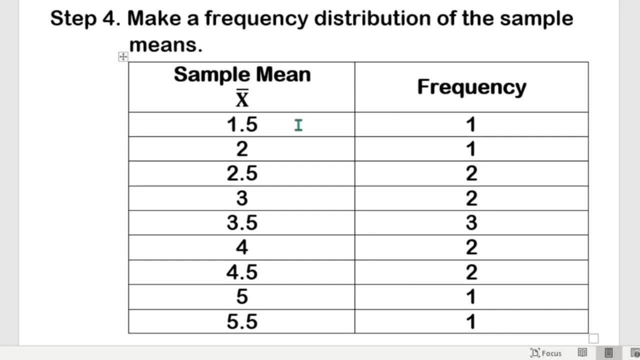 This table is already the sampling distribution of the sample means Because, as the definitions say, says that the sampling distribution of the sample means is simply the frequency distribution table using the means of all the possible samples. and we have it here. But remember that we have a random variable and a random variable. 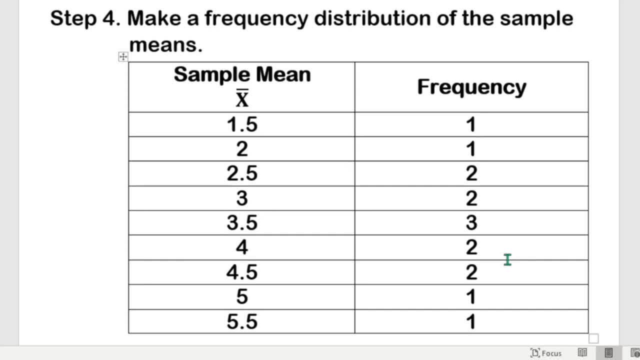 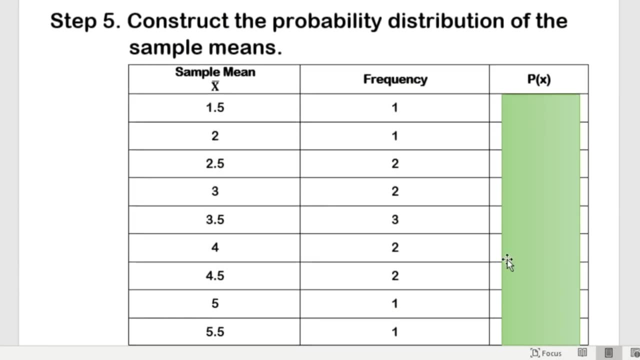 has a probability distribution table. The sampling distribution of sample means is also called the probability distribution of sample. To construct the probability distribution of sample means, we proceed to step 5.. Now, as you can see in our table here there are three columns. Again, the first two columns. 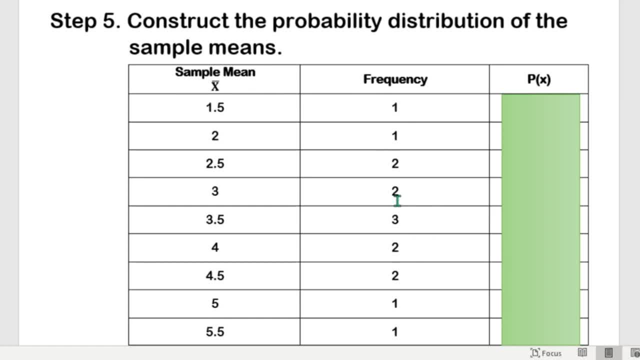 represent simply the sampling distribution of the sample means. You have the sample mean, the frequency. Now we only add one column which will label us as the sample type, the p of x or the probability of each sample mean, That is, the probability that the sample mean is. 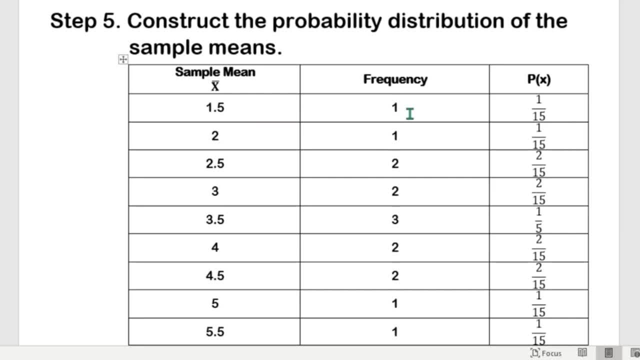 1.5 is 1 out of 15.. We refer to the frequency to be able to get the probability, Because there are 15 possible samples. then we have our 15 as the denominator. here Again, the probability that the sample mean is 2.. We have 1 out of 15.. The probability that the sample mean is 2.5.. We have 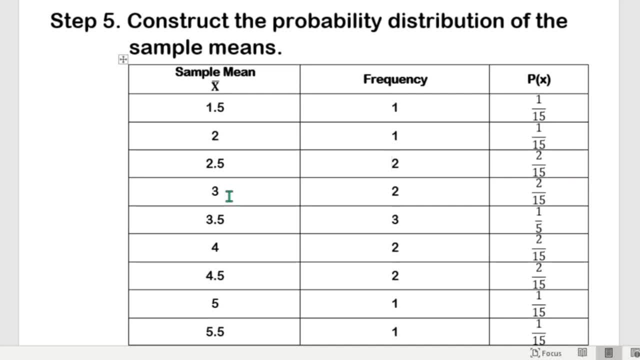 2 over 15.. The probability that the sample mean is 3.. We have 2 over 15.. The probability that the sample mean is 3.5 is 3 over 15.. In simplest form, we have 1. fifth And the probability that the 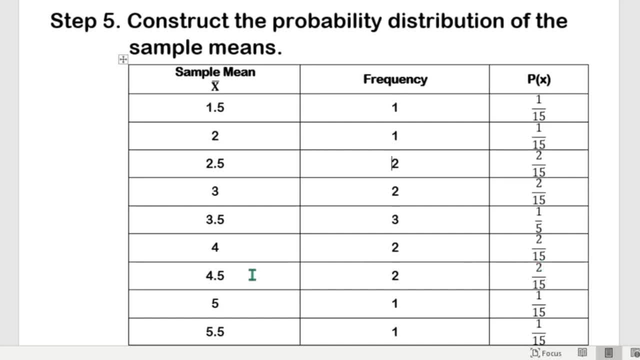 sample mean is 4 is 2 over 15.. The probability that the sample mean is 4.5.. We have 2 over 15.. The sample mean is 5. 1 over 15.. The sample mean is 5.5.. The probability is 1 over 15.. Now 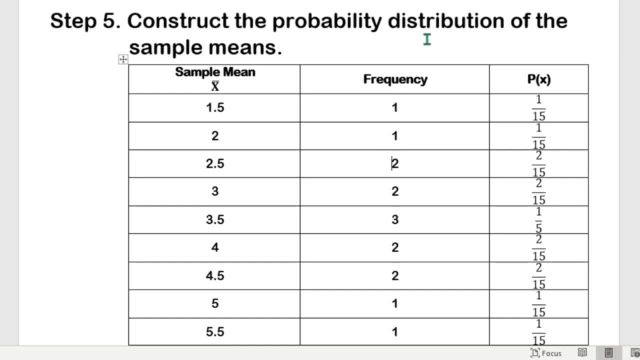 we have constructed the probability distribution of the sample means.